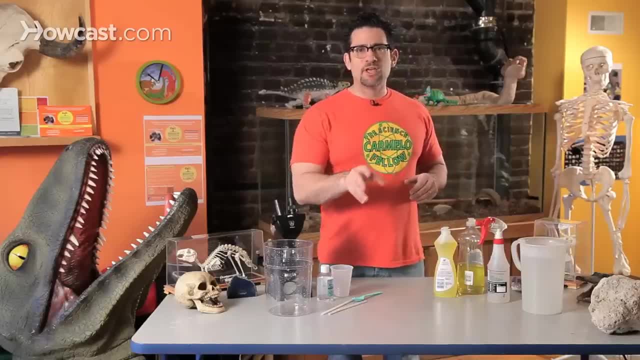 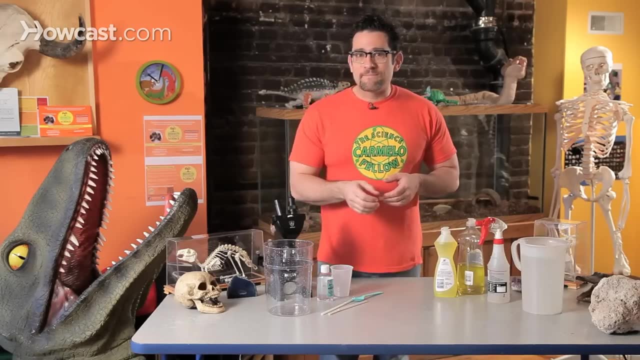 call this bubble-ology. You're all. everybody loves bubbles. If you're in the bathtub- and I love to take bubble baths, That's why my skin is so smooth- But think about it, You play with bubbles in the bath, right? 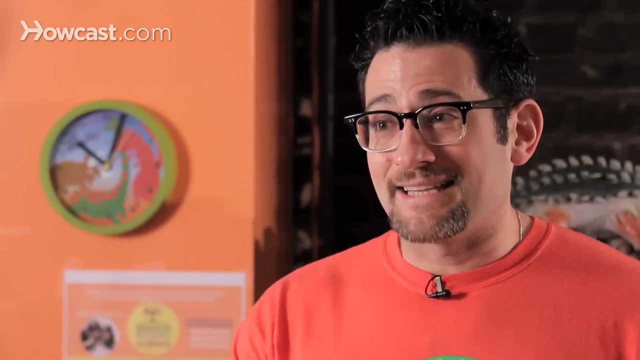 Or if you fart in the bath, you make a giant fart bubble. That's not that bad until the fart hits the top of the water and then it smells. That's a little disgusting, but you don't want to do those type of bubbles. 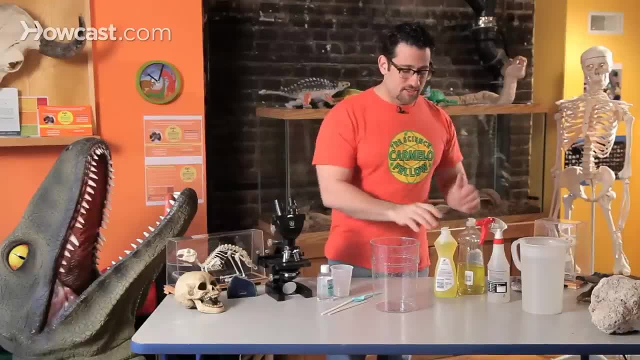 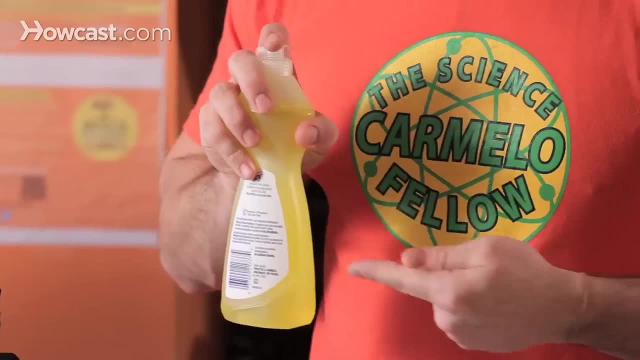 But right now, I'm going to show you how to do it. Right now, all I'm going to need is water, and you're going to have to use some of your parents' dishwashing soap. Okay, Keep it a secret, but it has to be dishwashing soap. 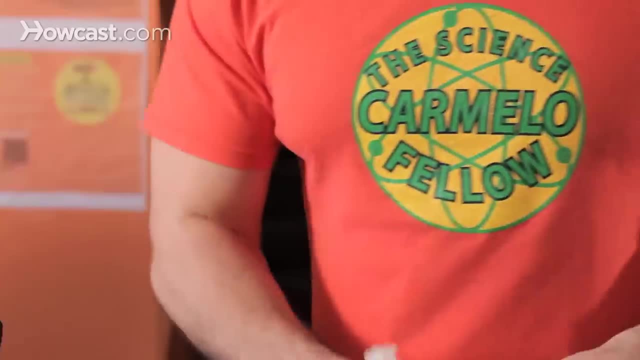 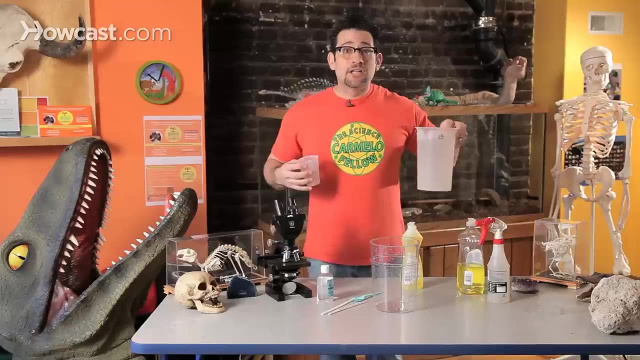 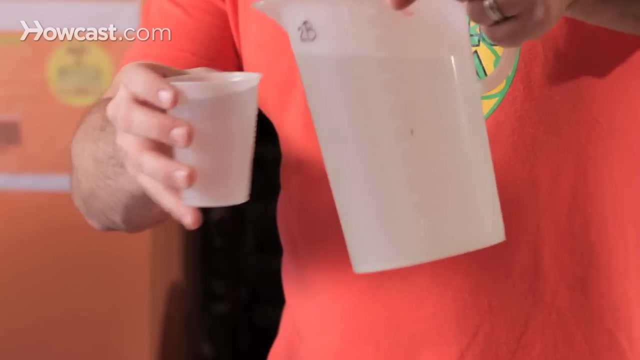 Not shampoo, not body wash, Dishwashing soap. And I'm going to show you what I'm going to do. Okay, First cup. I love you. see, science and math go hand in hand. Okay, I'm going to measure four cups of water, so you guys can count with me. 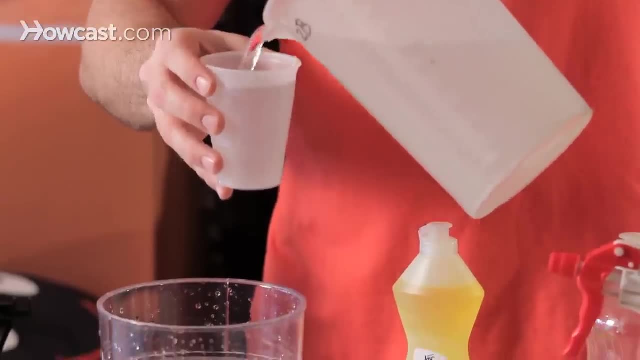 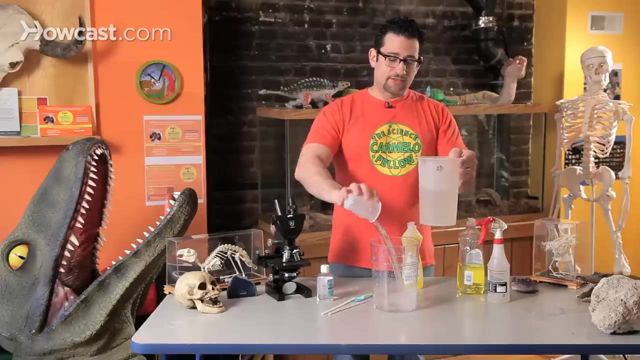 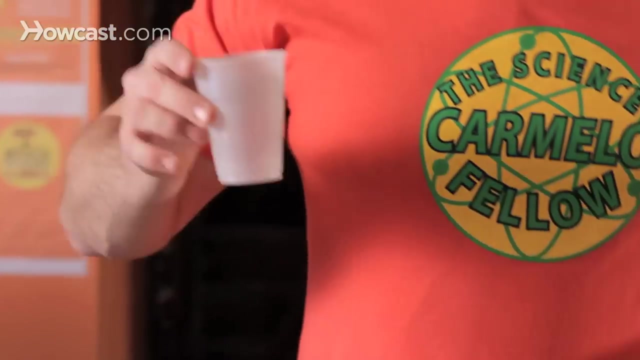 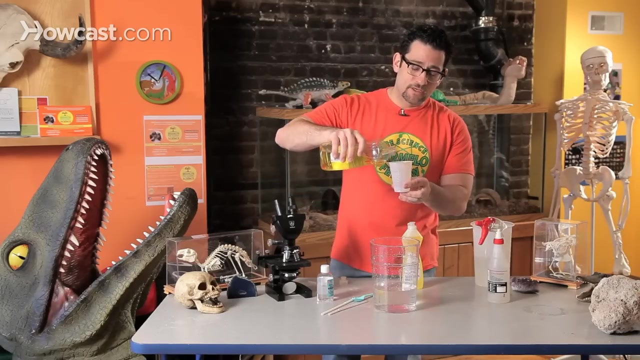 One cup, two cups, that's three cups, and that is my fourth cup, And I'm going to use half a cup of dishwashing soap. Okay, Just like this. I apologize, It does look like something. Okay, The other one's going to the bathroom. 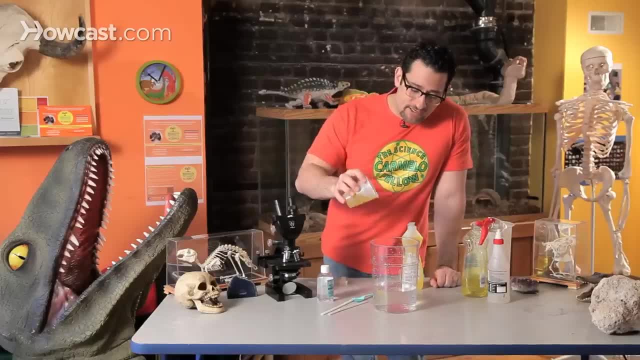 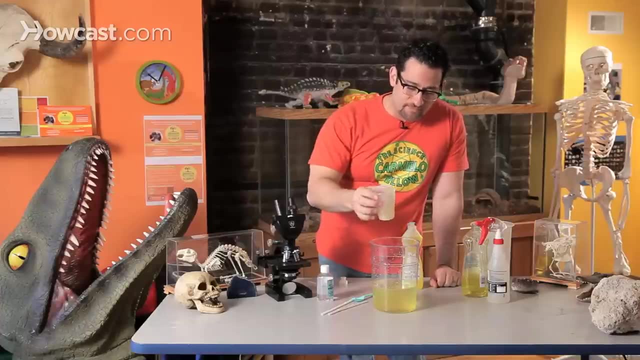 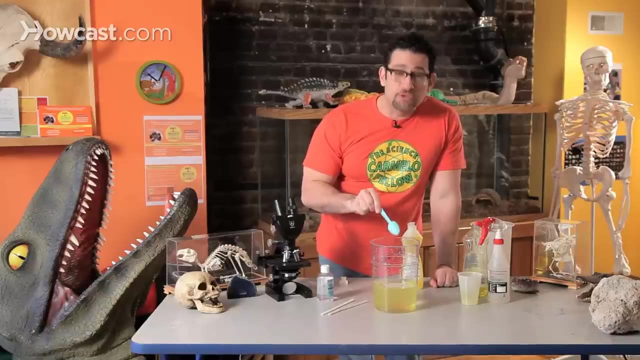 A little gross And I'm going to pour this into my container just like that, And I created a mixture, a soapy water mixture. Now I have a cool little secret for you guys. Okay, If you do not have my next chemical, you do not need to use it. 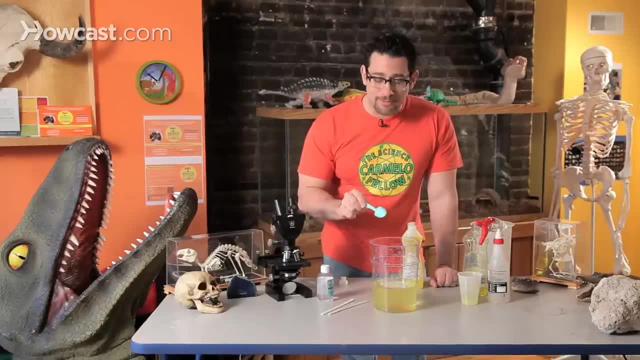 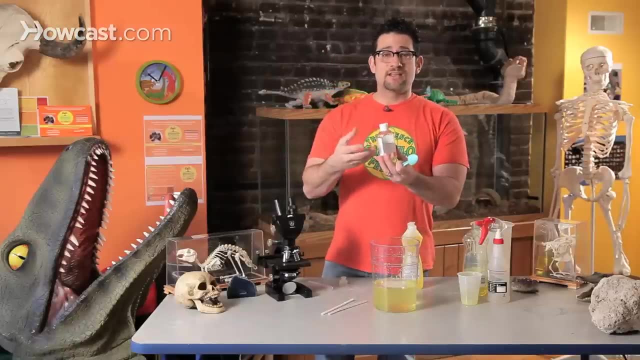 But when you go to the store, to the toy store, and you buy that special bubble solution, the reason why those bubbles do not pop as fast is because they're using a special ingredient that you can get at any pharmacy. Okay, It's not that expensive. 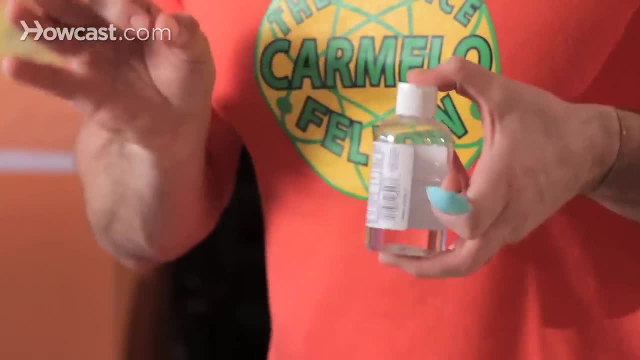 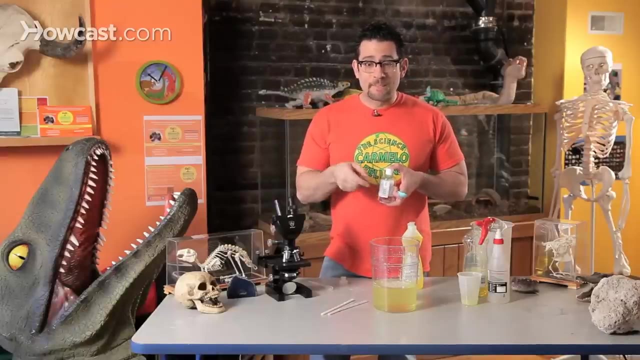 It's called glycerin. Glycerin will cause your bubble not to evaporate. You see, Bubbles are made out of water. When the sun heats up the water, think about if you have a spill on the floor, right? 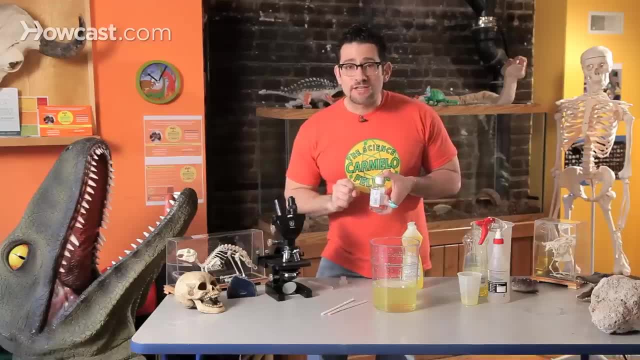 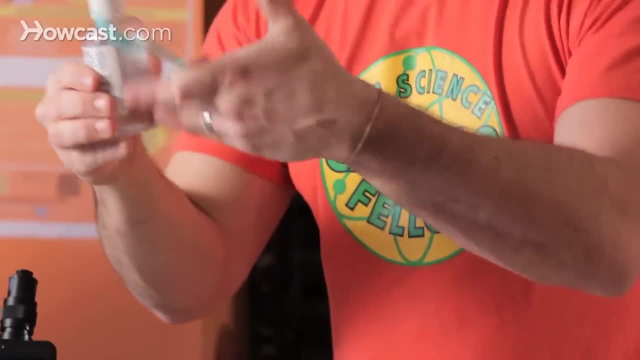 The spill is there. You go out to play. you come back, is the water still on that floor. No, it's not What happened to it. It evaporated, It turned into a gas that's all around you. Well, by adding glycerin, it causes the bubbles. 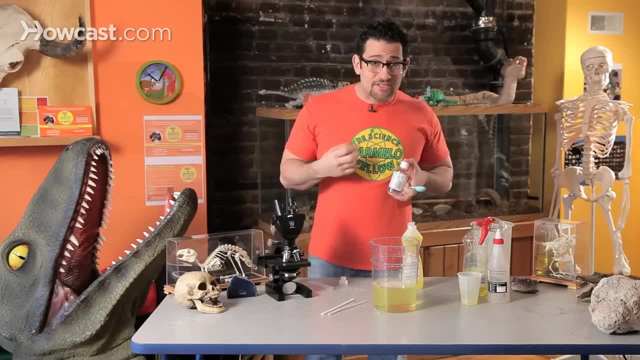 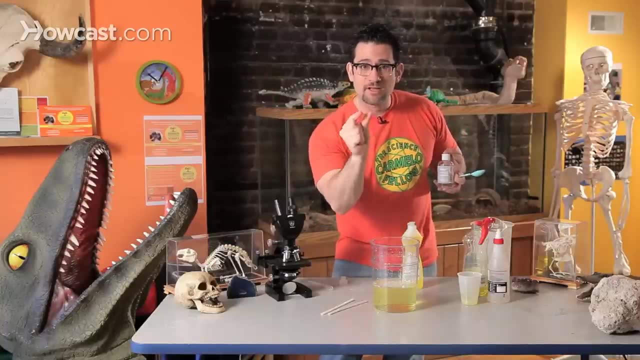 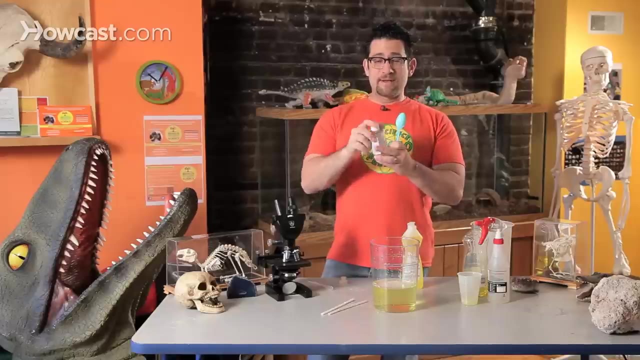 See, It's like skin. okay, Their skin is not like our skin. It's extremely elastic. It can stretch and stretch and stretch. I could take the smallest bubble. I could turn it into a bubble the size of this room. Bubbles have amazing properties, okay. 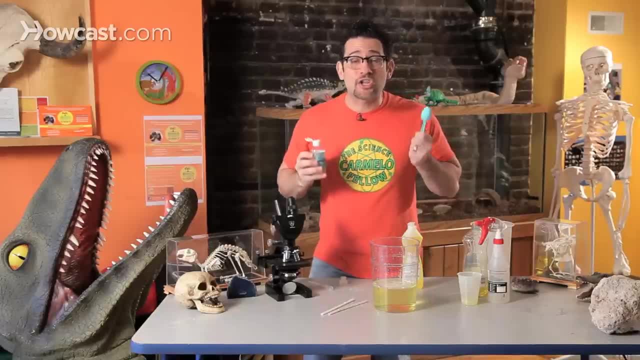 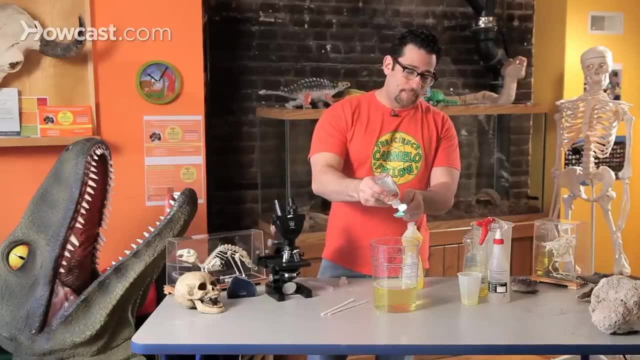 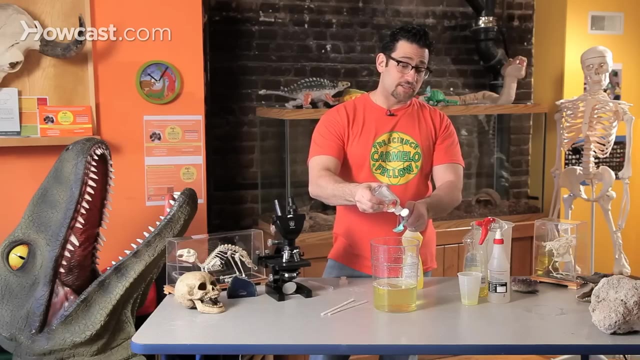 But now, by me adding this glycerin, it causes my bubble not to evaporate as fast. Remember, evaporates when liquids turn into gases. okay, So I'm going to put, let's see, One teaspoon of glycerin and again, you don't need to do this. 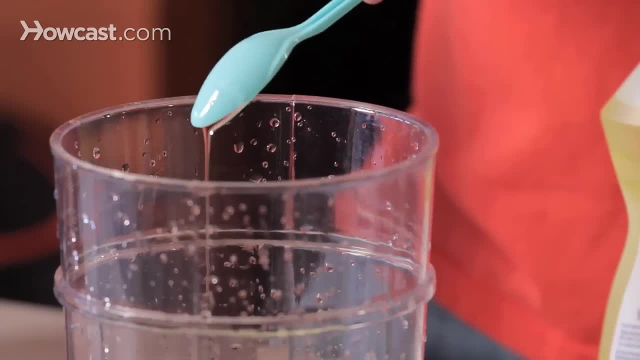 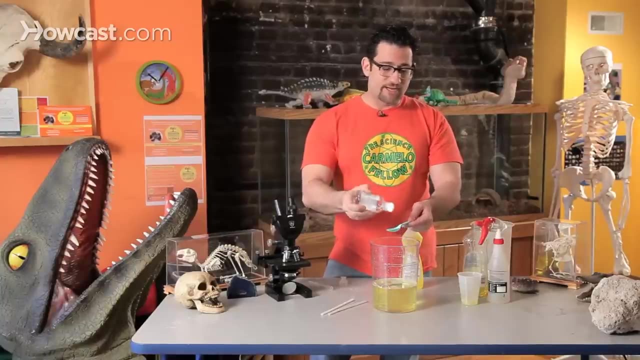 It'll still work without it, so you don't have to be upset. You all have dish washing. so because hopefully you wash your dishes and you all have water, this will just cause it not to evaporate as fast, And I'm just going to put four of these, okay. 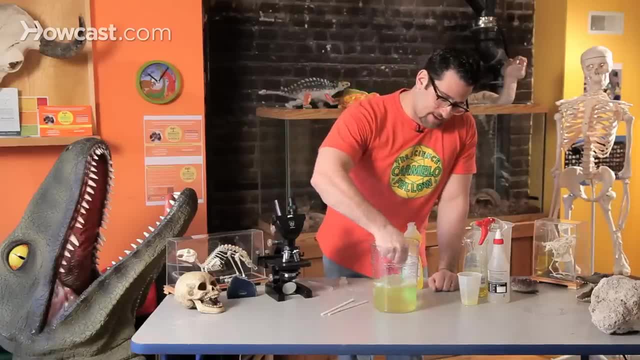 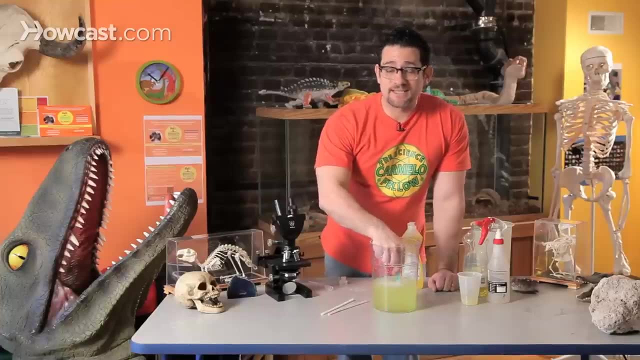 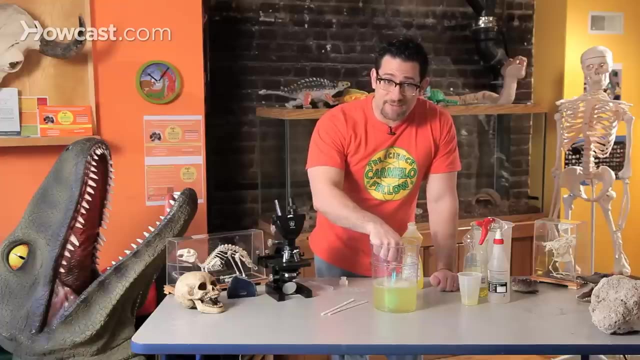 And then I'm going to stir it around And now I have created an amazing bubble solution. Now Some of you are going to say to me: Carmelo, what does this have to do with how we started? You started talking about matter and I told you that matter takes up space and I said: 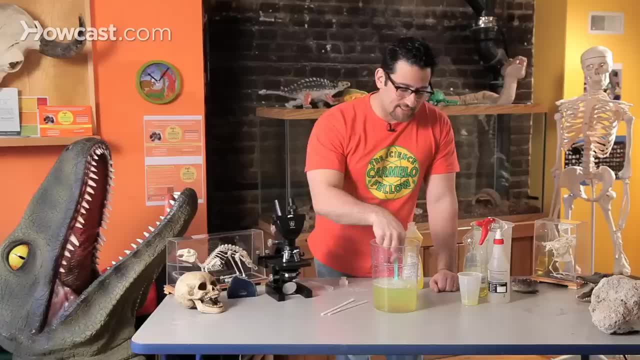 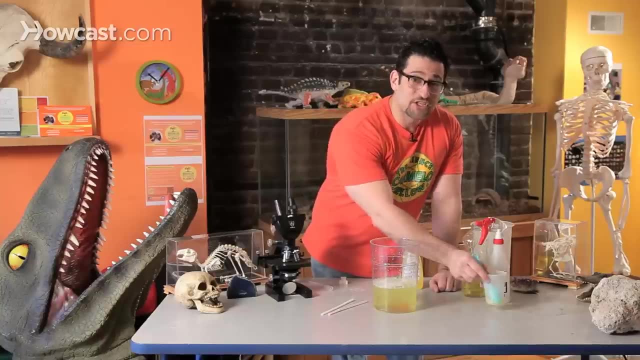 that there were three states of matter right: Solids, liquids and gases. And I then said: how hard is it to show you that gases take up space? Well, I can show you now. Check this out, okay, You see. 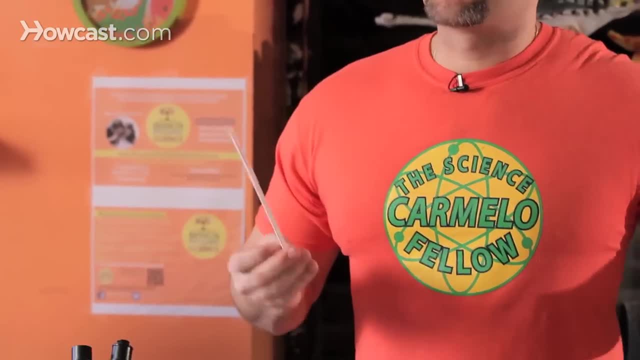 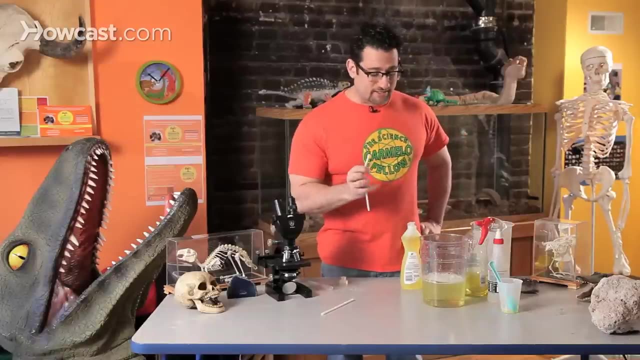 All I need now is a straw. Now some of you are going to be like: oh man, this is boring, The dude's going to blow bubbles in the air. I've been blowing bubbles in some too, But wait, We're going to do this with a twist, okay. 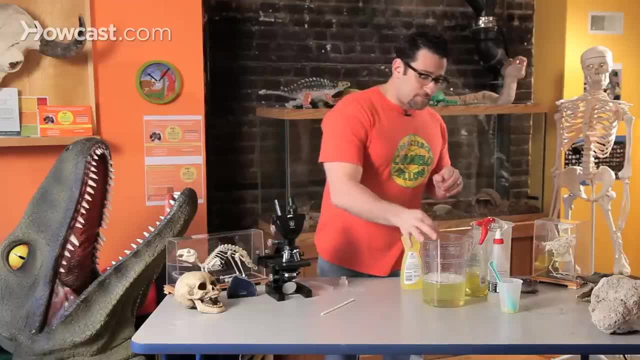 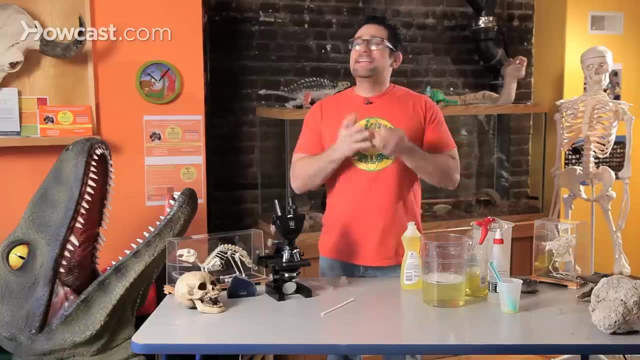 Take your straw First. I do need to show you something, okay? Because if you dip the straw in and you take the straw out and you blow hard, you killed the bubble already. You didn't even have a chance to become a bubble. 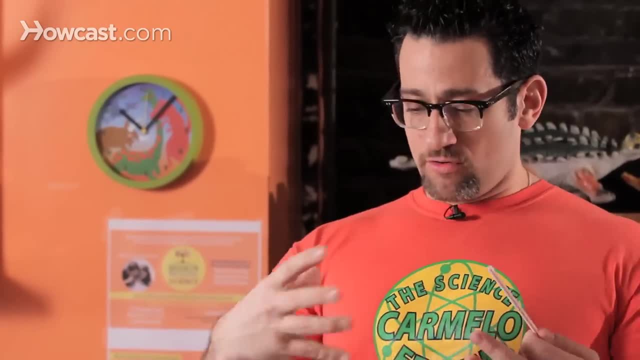 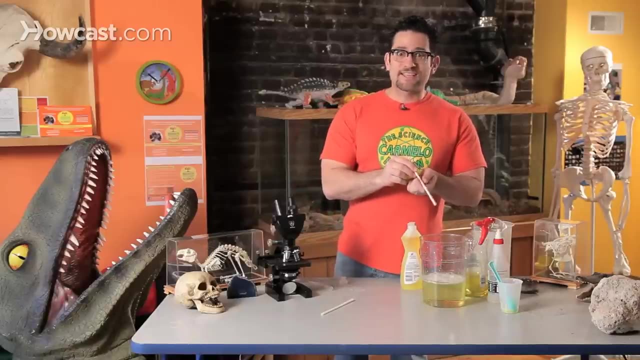 The bubble's dead. You want to blow slow. Now you have a force of air. Your lungs is your source of your air. So when you dip your straw in and you take your straw out, sounds like the hokey pokey. 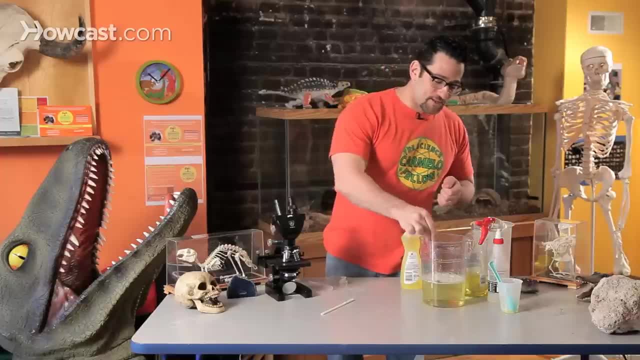 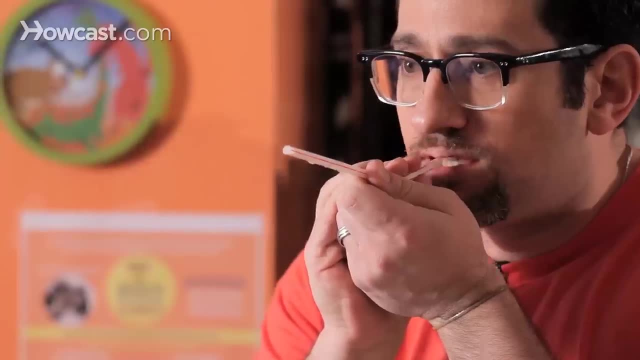 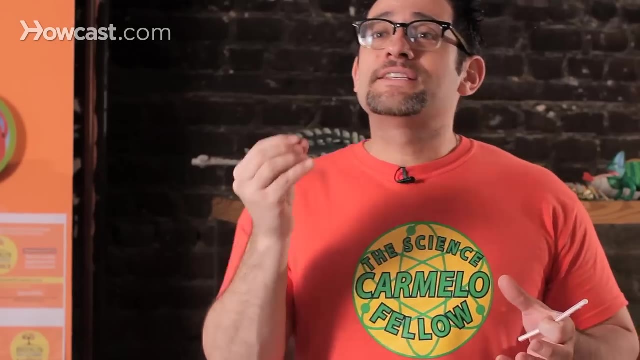 Dip your straw in and you take your straw out and you do. No, All right, Dip it in, take it out and blow slow And it pops. Actually, it evaporated, Did you see? The more air I put, the bubble got bigger. 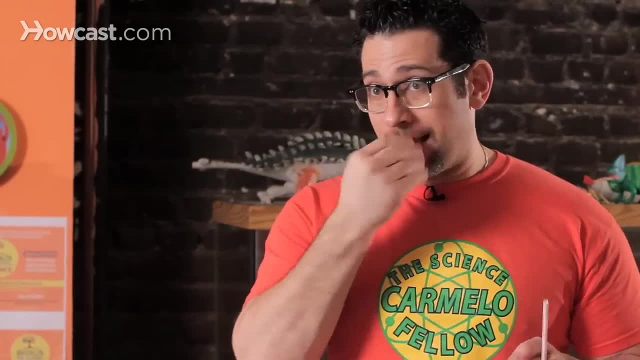 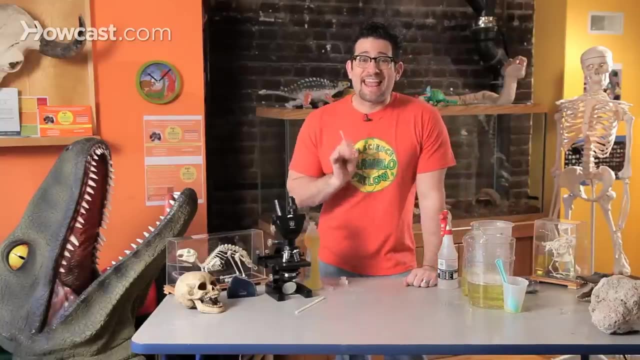 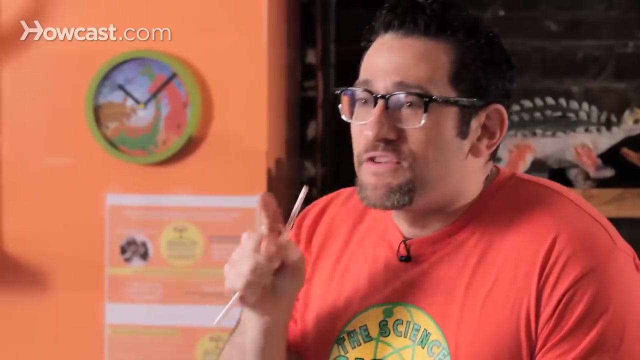 This is proof that air and gas does take up space. But how about this? I said we're going to do it with a twist. Bubbles have an enemy. It hates things that are dry. If a bubble touches something dry, the bubble will go bye bye. 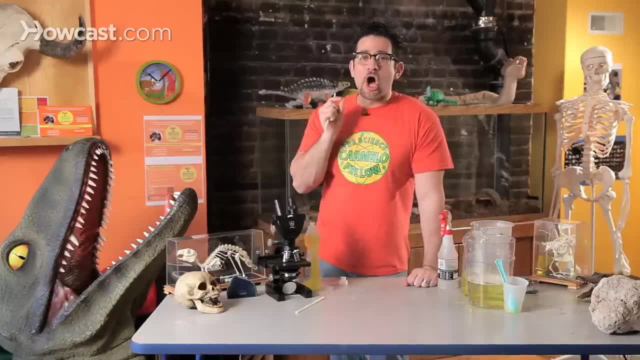 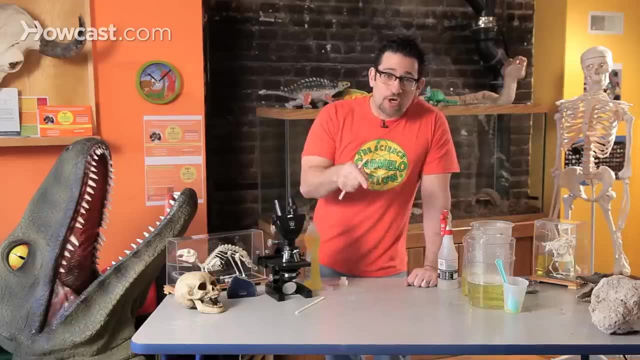 But if you wet anything, you can make a bubble on anything, Because bubbles love things that are wet and they won't be upset. But remember, if it touches something dry it will go bye bye. If you don't believe me, check this out. 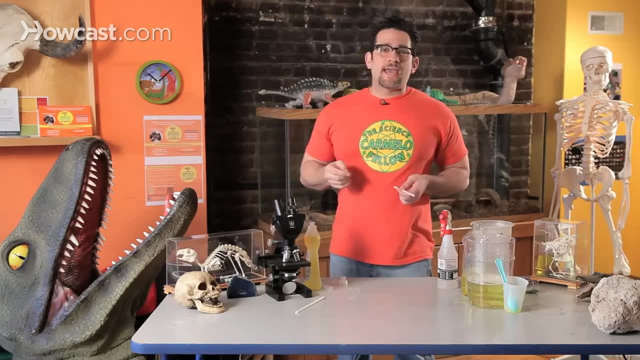 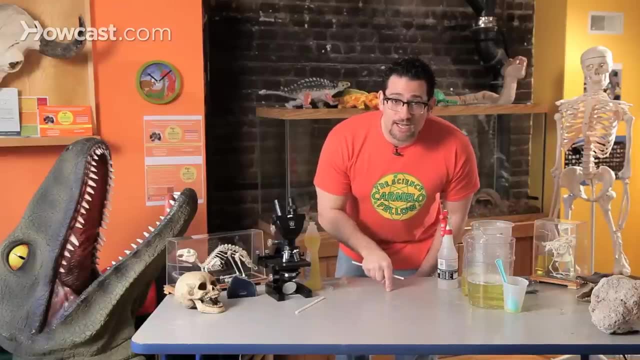 See my table. It's dry. See, everybody blows bubbles into the air. You can blow a bubble on anything, But if you blow it, it popped Right. Table's dry. If it blows, bye, bye. But watch this. 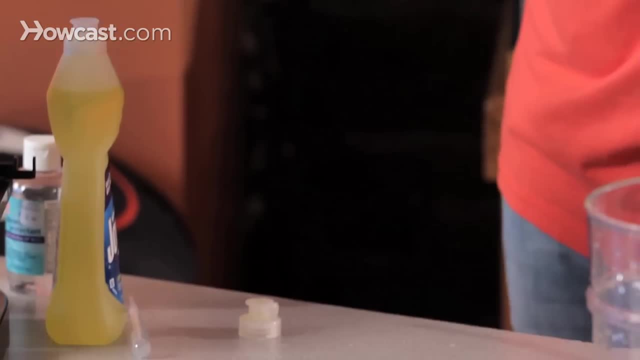 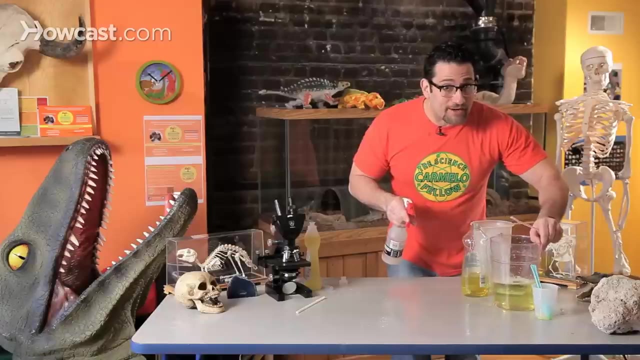 If I wet the table a little spray, I'm going to wet the surface of the table. The more the table's wet, the bigger I can get my bubble. But the moment that bubble touches a dry spot on that table, that bubble will pop. 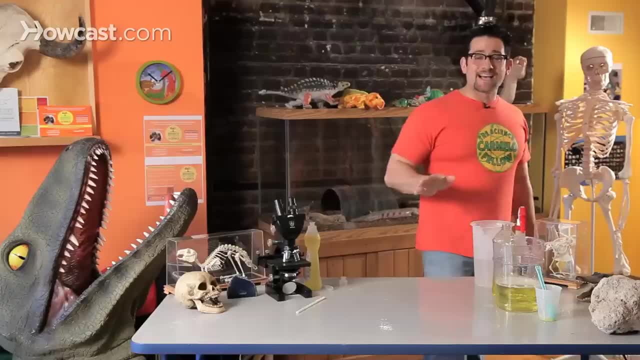 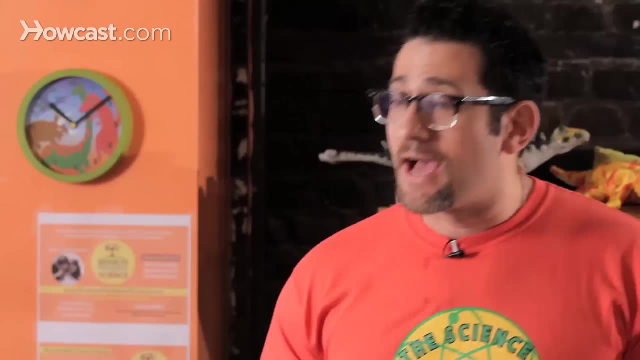 Now, believe it or not, I can make a bubble the size of this entire table. I just need to put more what Gas? The more gas, the more space. I put gas, the more space. This is proof that gases take up space. 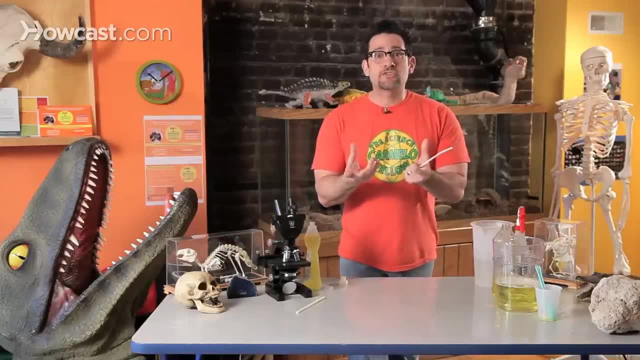 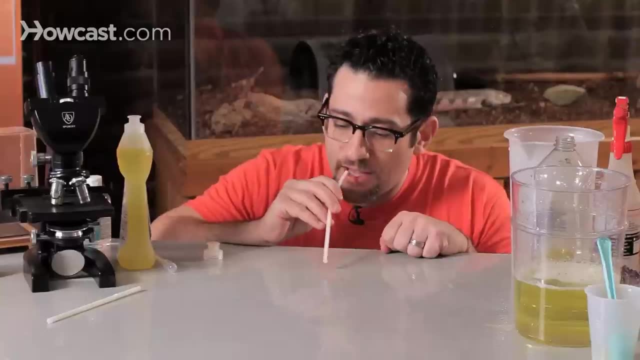 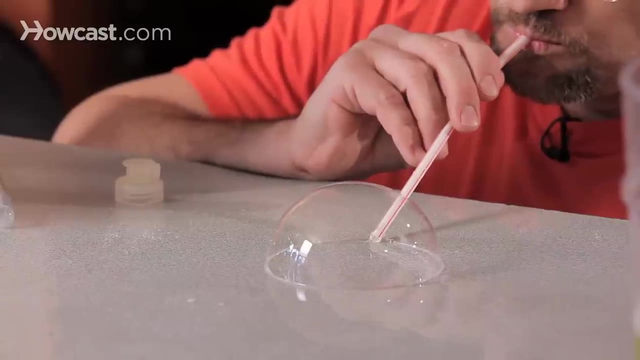 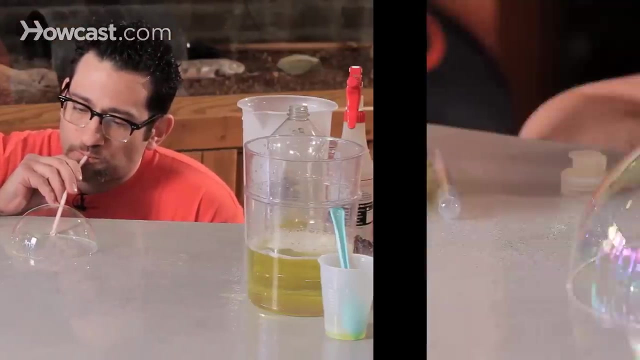 It's just so cool how you can use bubbles and water to illustrate that air takes up space. Dip your straw in, take your straw out and now observe the master. Check this out. I'm going to keep blowing until it pops. Look at that. 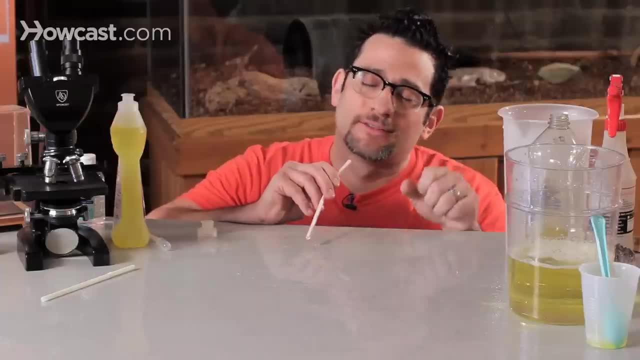 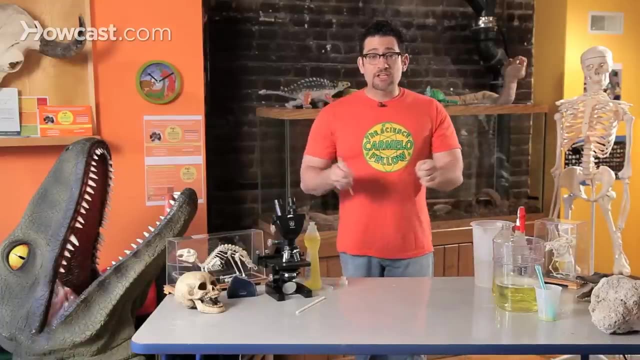 Think about how small the bubble skin was inside the straw. Ugh, It evaporated. Now, once it evaporates, you know what's cool? It leaves a perfect circle on your table. You can take a ruler and you can do like a bubble Olympics. 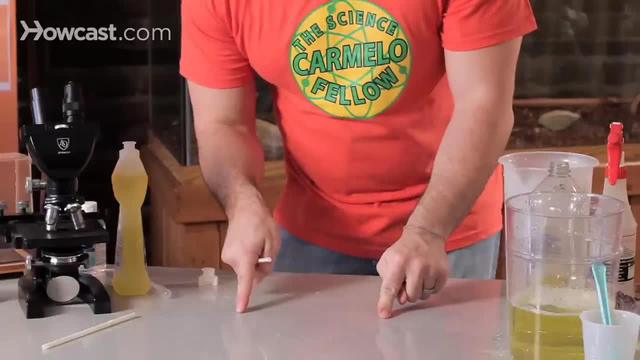 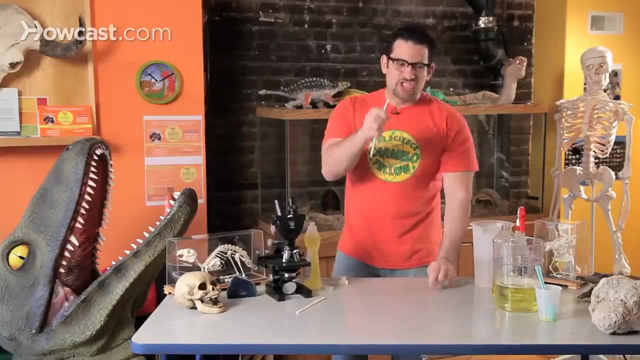 Challenge yourself or challenge your friends. Measure the diameter of your bubble, Okay, And you can be like, wow, That was eight inches. Well, now try to make it ten inches. And you want to see something even cooler? Check this out. 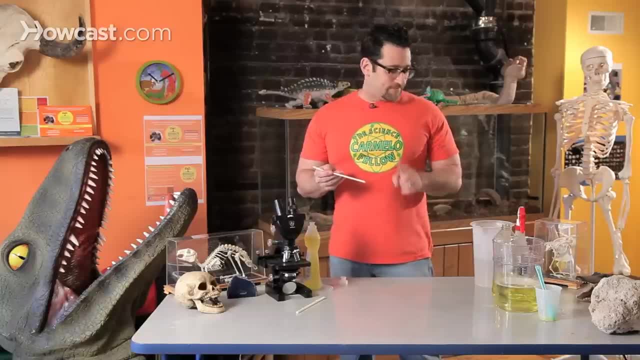 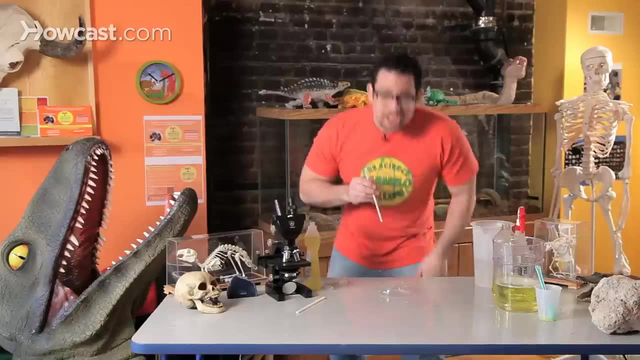 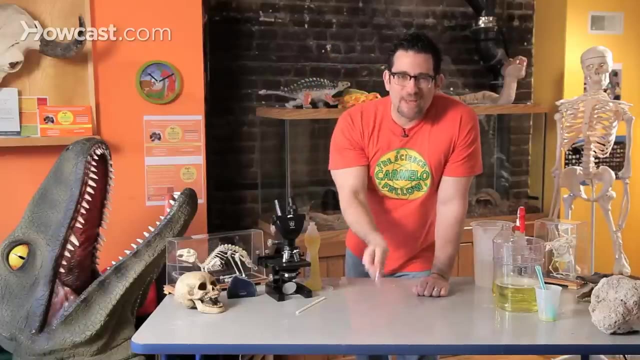 Okay, What happens if you touch a bubble? The bubble's going to pop right. Watch this. Make a bubble. Now, if I touch it with the dry part of the straw, that's not wet bubble pops, But I can actually cut a bubble with a knife or with a straw or with a scissor, as long 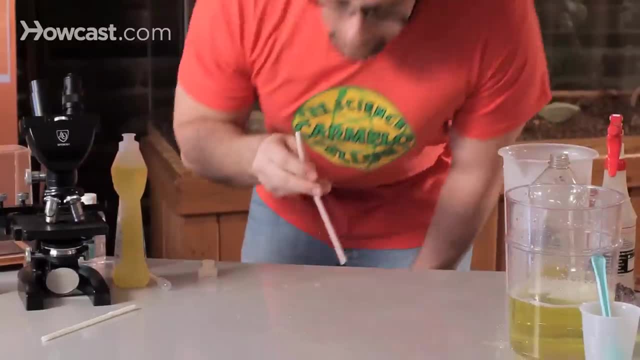 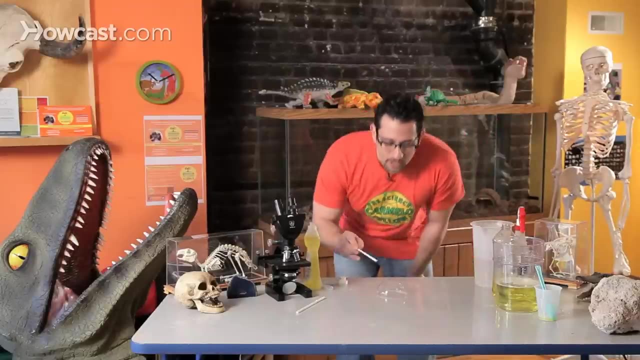 as it's wet. Check this out. Make a bubble. Wet my straw, Look I could cut it. The bubble doesn't pop. But the minute you touch it with something dry bubble pops. Saw that. I want to see something even cooler. 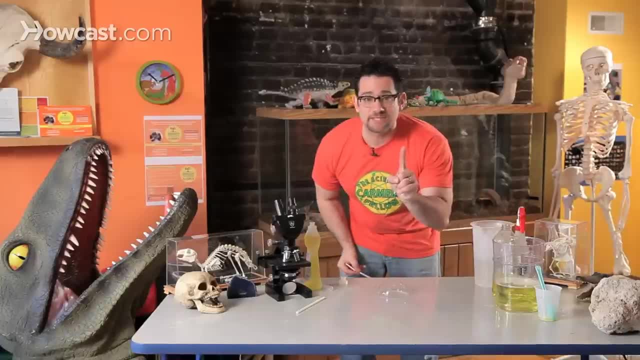 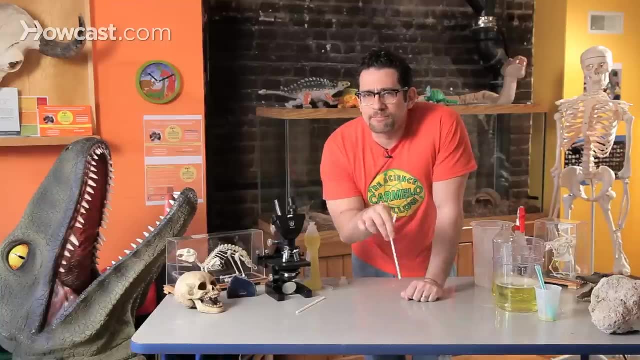 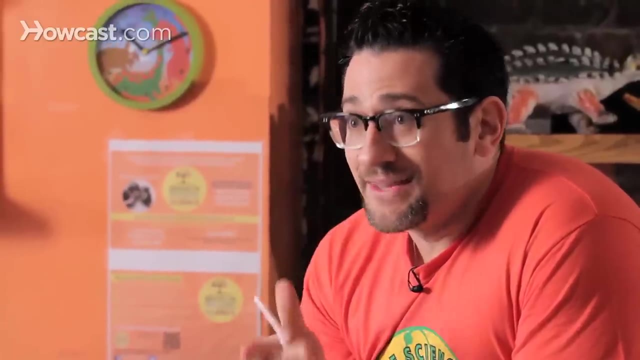 If I'm able to put my straw in a bubble. see, this is all about what science is. It's about asking questions. Ask a question and then you make a prediction, And then you test your prediction to see what happens. Well, if I'm able to put my straw in a bubble, what happens if I blow? 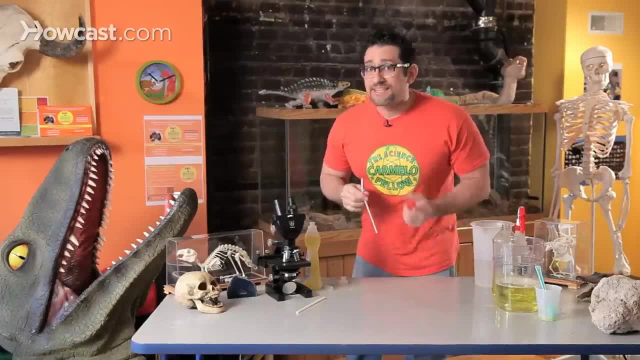 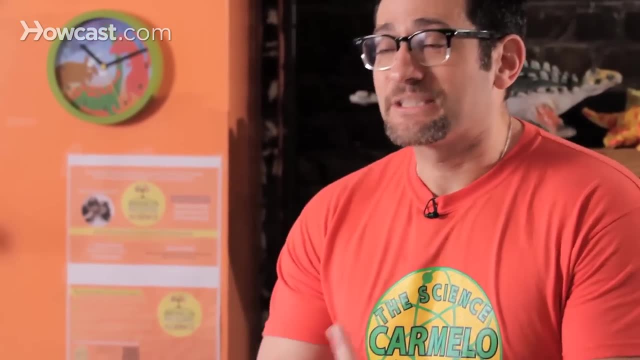 Another bubble in a bubble? That's the question. Now, my prediction is: hmm, maybe the bubble will get bigger. Now I'm going to test it. That's the process. I'm going to do it now. Well, so let's see. 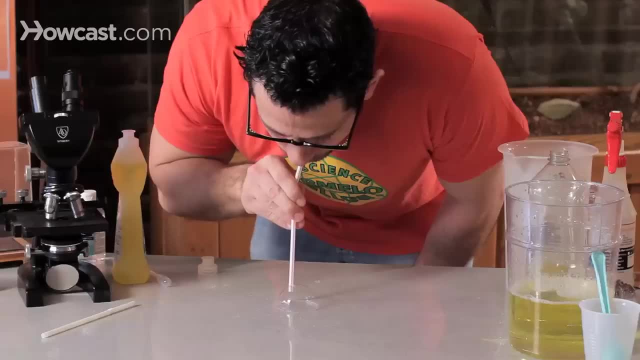 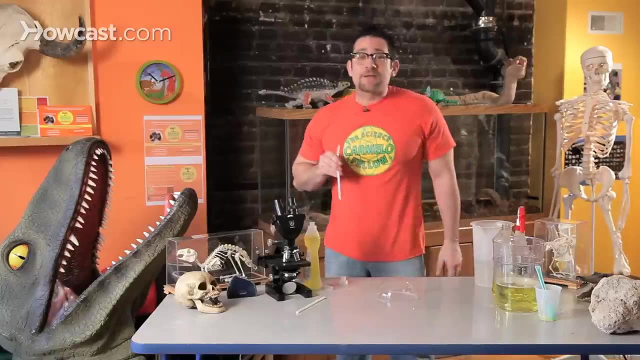 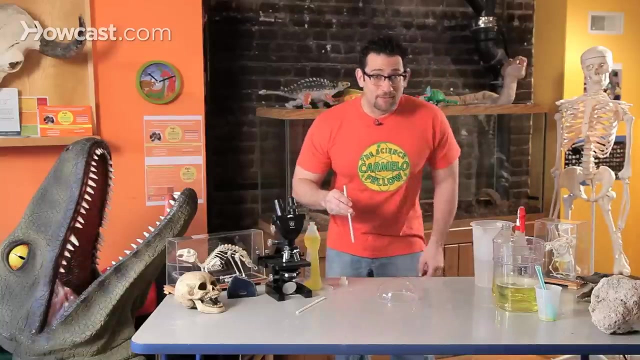 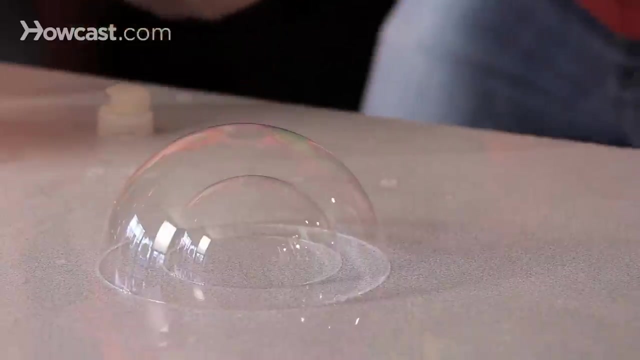 I'm going to make a bubble. Now I'm going to make a bubble, Or see what happens if I dip this back in my solution. What happens if I blow another bubble? What happens if I blow another bubble in a bubble? I just made a bubble inside of a bubble. 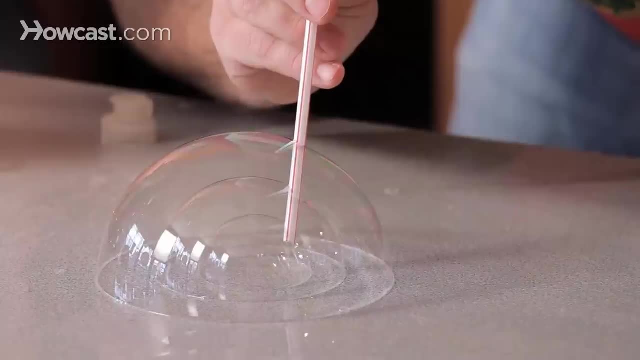 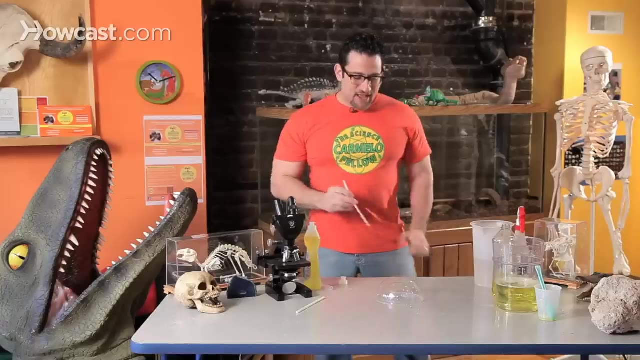 Can I make a bubble in a bubble in a bubble? Whoa? Can I make a bubble in a bubble in a bubble in a bubble? Oh my gosh. Now you can ask another question: What happens if I touch the outside bubble? 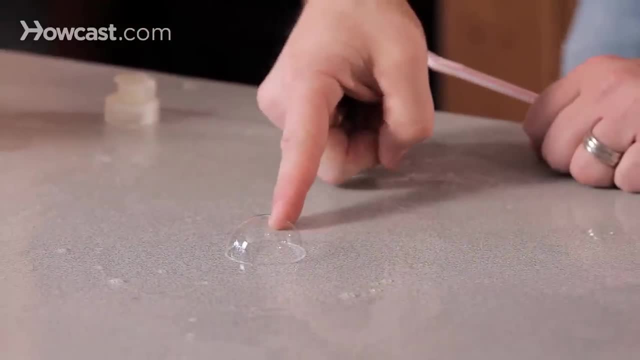 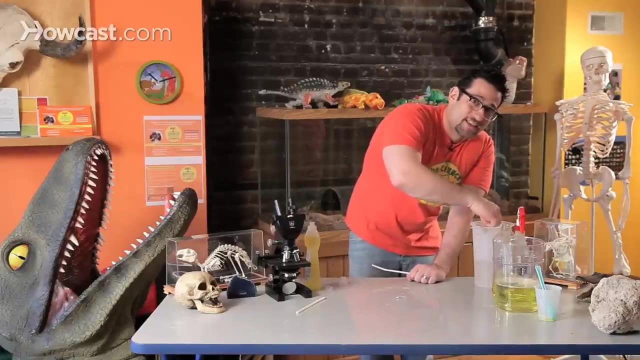 Make a prediction. Test it: Pop, pop, pop. Look at the baby bubble. Wait, do you think I could pick up that bubble? if my hands are dry? Probably not. What if my hands are wet? Can I pick up a bubble? 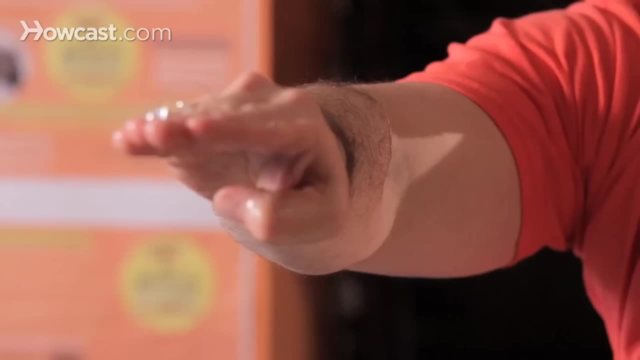 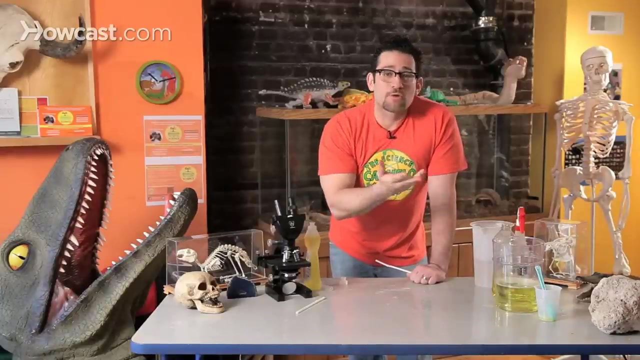 Oh, I got them. Think about how much fun you can have. We could prove that air takes up space and just have so much fun using nothing but soap and water. And that's my bubble-ology experiment. 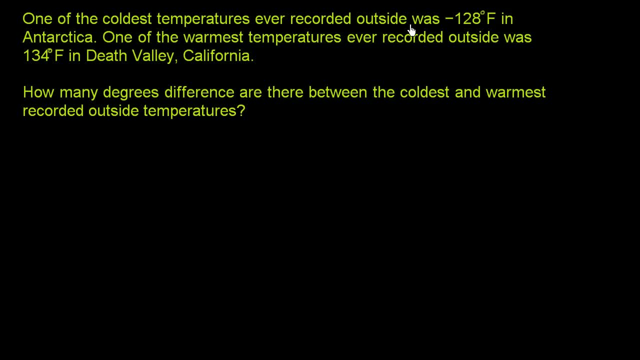 One of the coldest temperatures ever recorded outside was negative 128 degrees Fahrenheit in Antarctica. One of the warmest temperatures ever recorded outside was 134 degrees Fahrenheit in Death Valley, California. How many degrees difference are there between the coldest and warmest recorded outside temperatures? 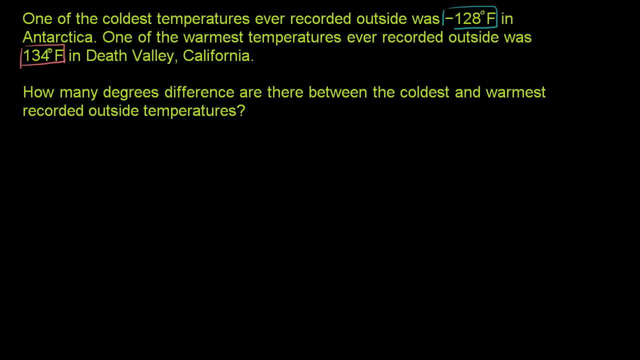 So let's think about this a little bit, And what I'll do is I'll plot them on a number line. But I'm going to plot on a vertical number line that has a resemblance to a thermometer, since we're talking about temperature. 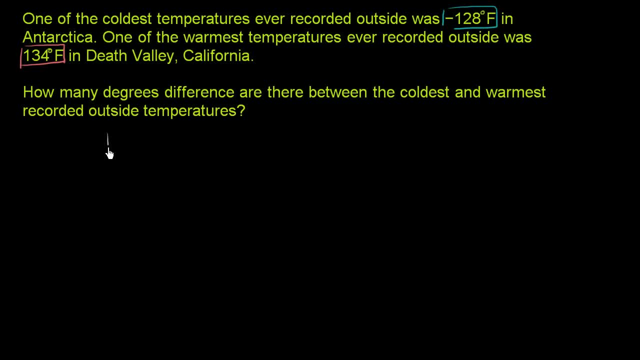 So I'm going to make my number line vertical right over here. So there's my little vertical number line, And this right over here is 0 degrees Fahrenheit, which really is of no significance. If it was Celsius then we'd be talking. 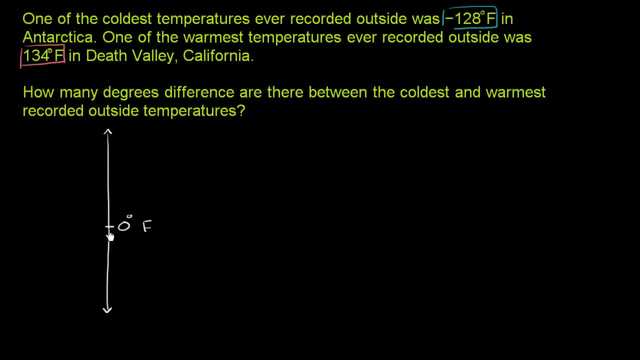 about the freezing point, But for Fahrenheit that happens at 32 degrees. But let's say this: This is 0 degrees Fahrenheit, And let's plot these two points. So one of the coldest ever recorded temperatures was negative 128 degrees Fahrenheit. So let's say that's right over here. This is negative 128 degrees Fahrenheit And one of the warmest temperatures ever recorded was 134 degrees. This is a positive 134.. So it's about that far and a little bit further. 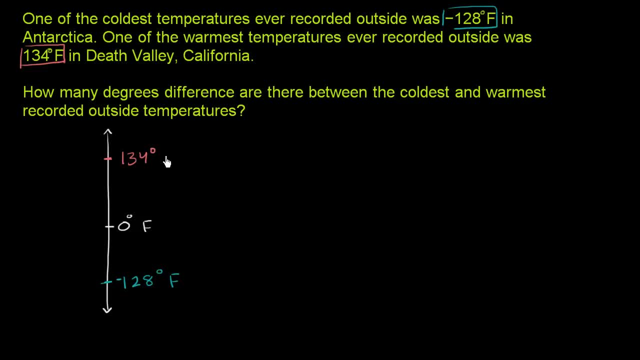 So it's a positive 134.. 334 degrees Fahrenheit. So when they're asking us how many degrees difference are there between the coldest and the warmest, they're essentially saying, well, what is this distance between the coldest and the warmest right over here? 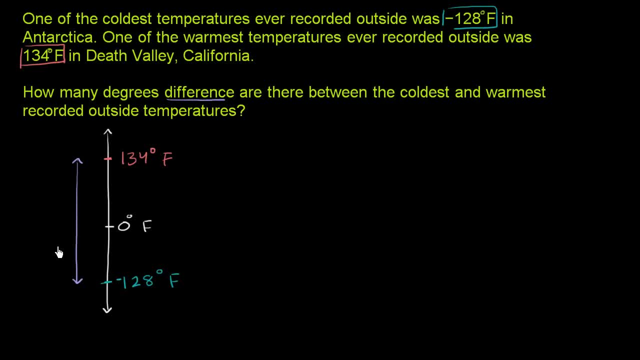 What is this distance? And there's a couple of ways you could think about it. You could say: hey, if I started at the coldest temperature and I wanted to go all the way up to the warmest, how much would I have to add? 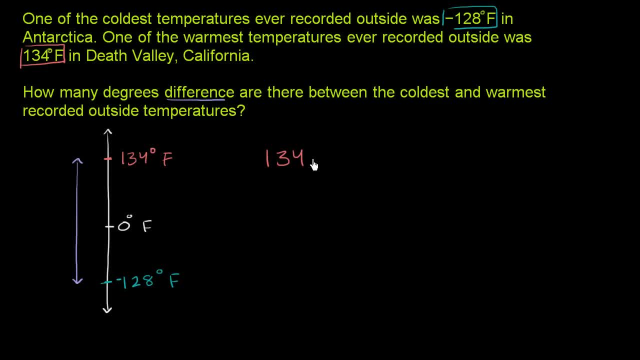 And from that you could subtract the smaller number, which is negative, 128.. So this is essentially saying what's the difference between these two numbers? It's going to be positive because we're subtracting the smaller one from the larger one.